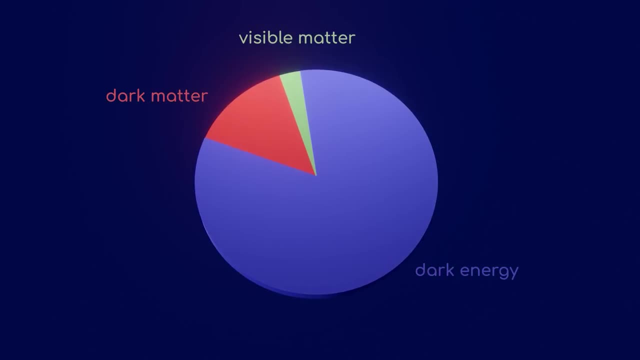 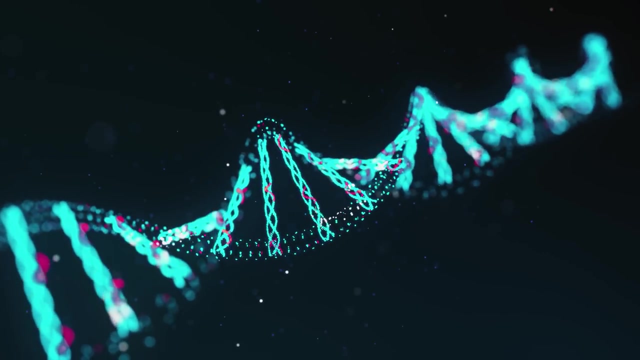 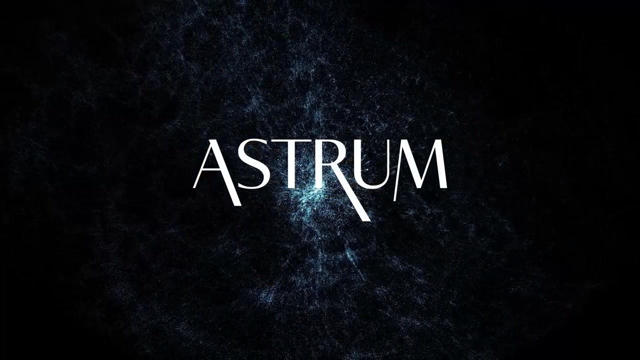 galaxies could never have come to exist, let alone life and humans. So how did the universe avoid this fate And how are we alive to even ask these questions? I'm Alex McColgan and you're watching Astrum. Join me today as we continue to learn. 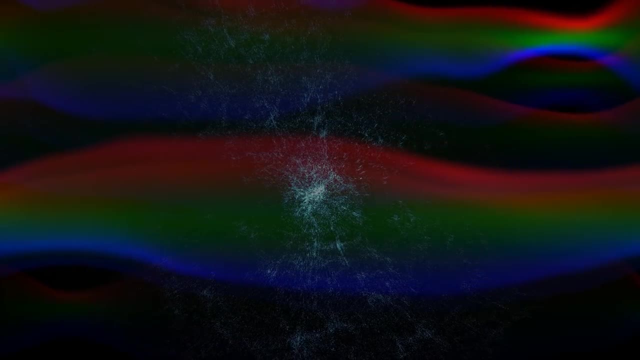 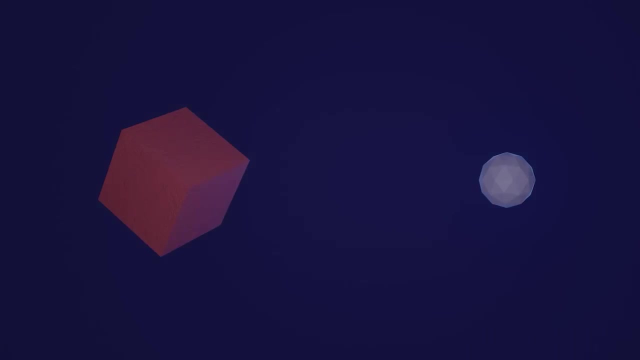 about the effects of dark energy on the cosmos and explore the maths that claims we really shouldn't have existed at all. One of the first things you might learn in a physics class is that gravity is an attractive force between two objects whose strength is proportional to each of their masses. Gravity- 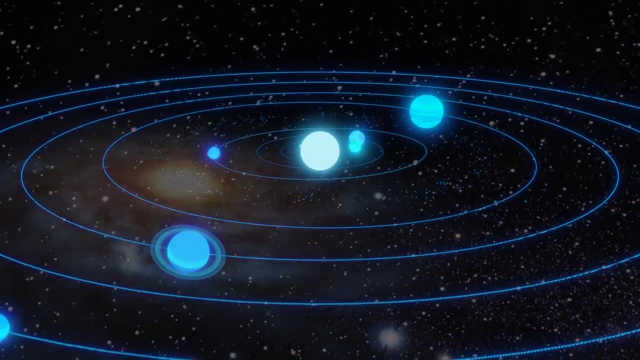 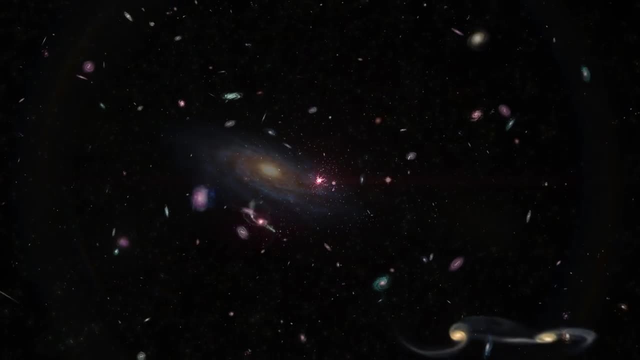 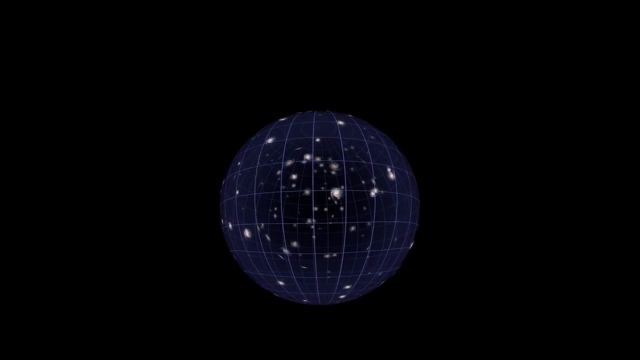 keeps planets locked in orbit around the sun, it keeps stars grouped together in the Milky Way, and it even attracts galaxies together to form galaxy clusters and superclusters. But if we zoom out further, This gravitational attraction begins to act in reverse, causing galaxy clusters to accelerate. 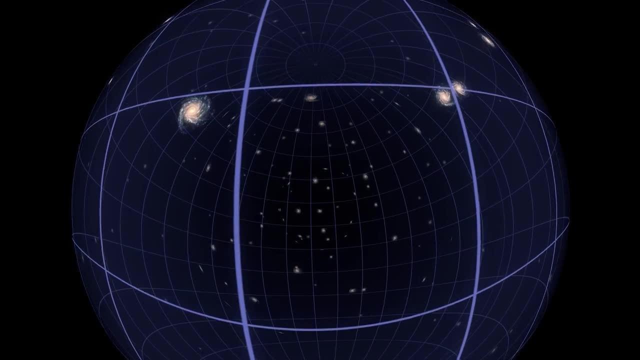 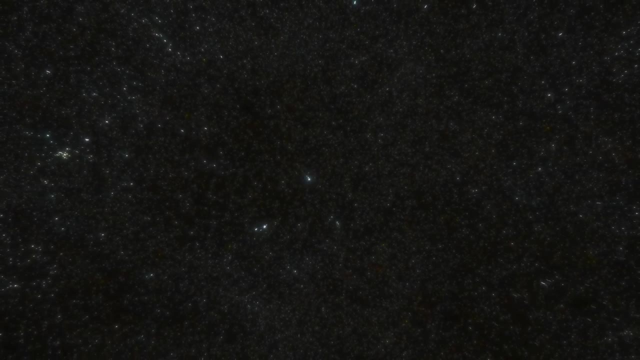 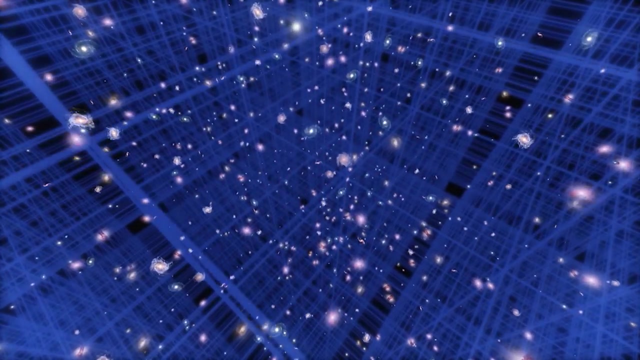 away from each other rather than drawing each other in. So what's going on here? Einstein's theory of general relativity gives us a lens through which we can understand this strange behaviour. In general relativity. space isn't just some background in which 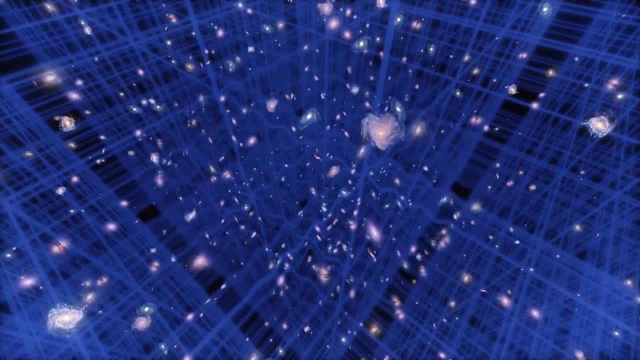 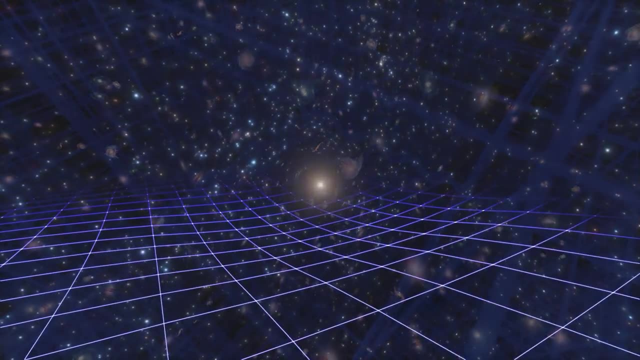 other things can move around Instead, space itself can move around. Space itself can move around. Space itself can stretch and warp and evolve over time. Einstein showed that in this framework, gravity is no longer a force, but rather a distortion of an object's 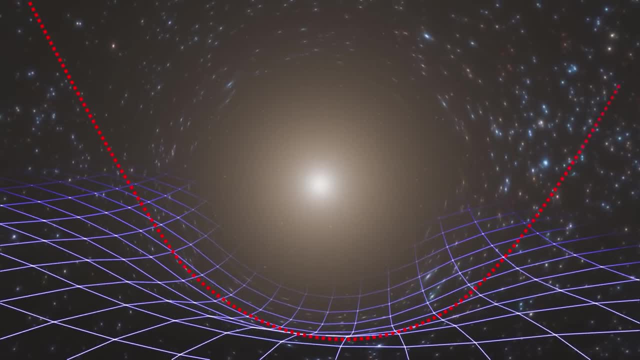 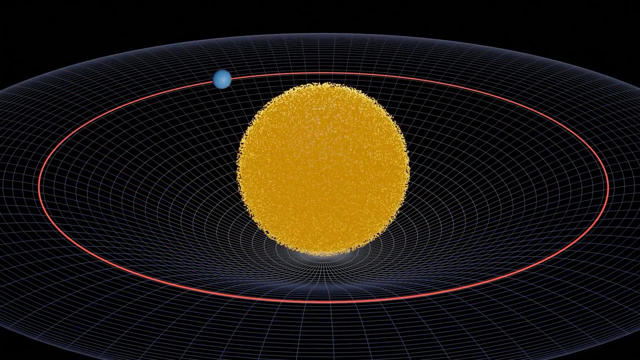 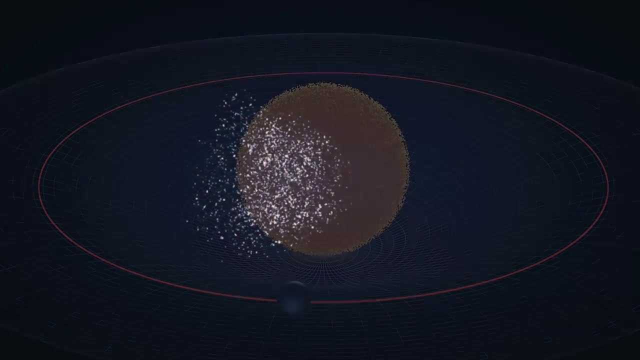 inertial path in a dynamical spacetime, For example when a planet orbits around the sun, in Einstein's description it's merely following a straight-line path in a curved space- means what we observe as a repulsive force between galaxy clusters should really be thought. 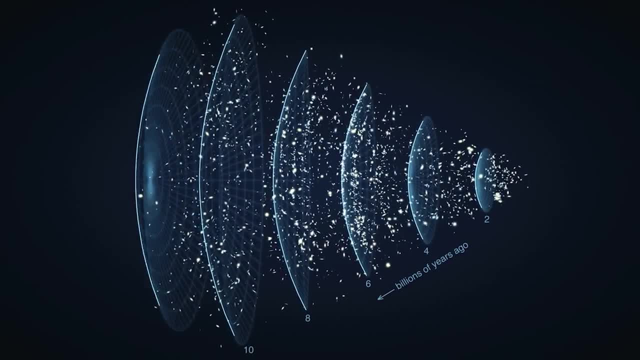 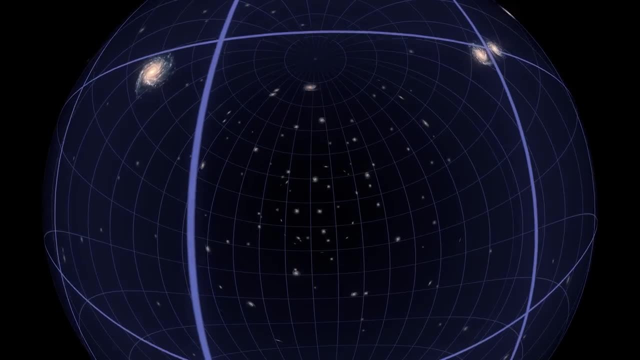 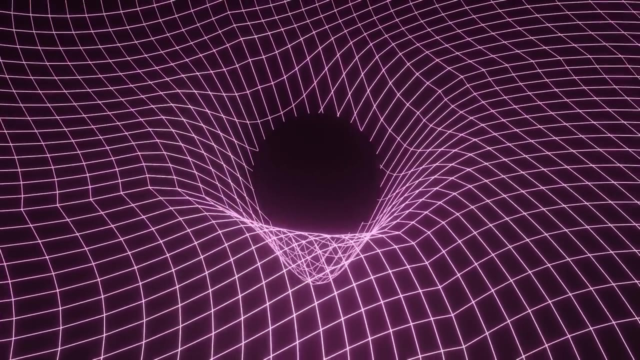 of as an accelerated stretching of the space between them. But what could possibly cause the expansion of space to accelerate like this on the largest scales of the universe? To begin to answer this question, we need to know what causes spacetime to stretch and warp. to begin with, In Newton's theory of gravity, all objects 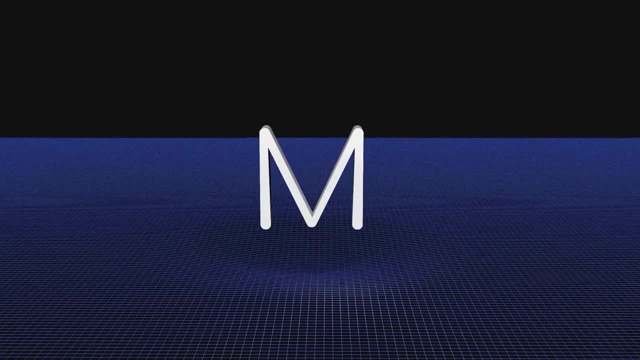 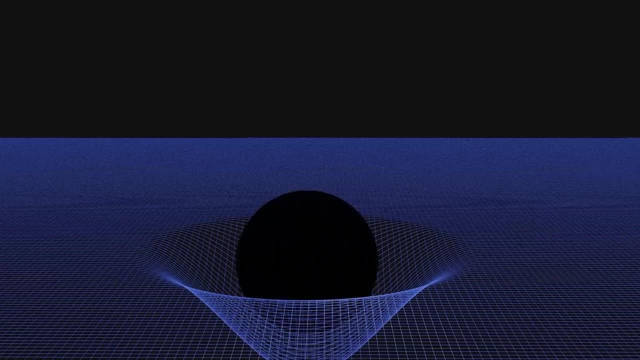 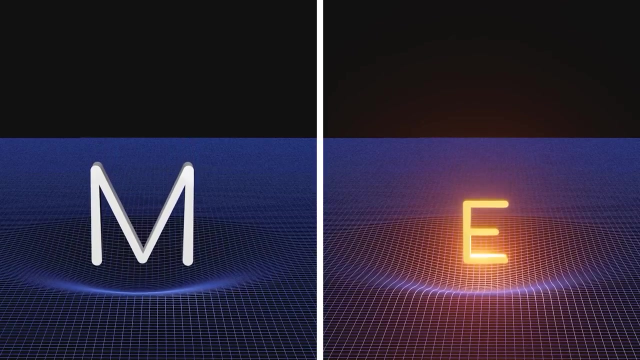 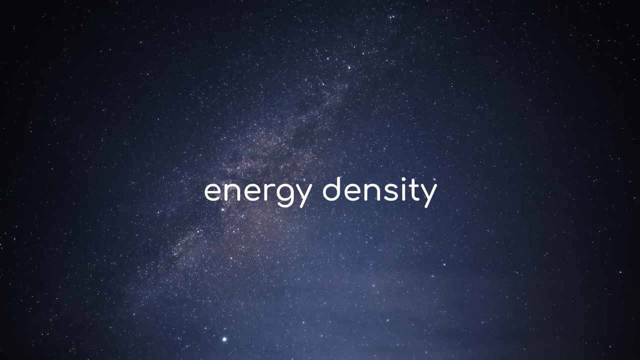 with mass exerted a gravitational pull And, in general relativity, all objects with mass curved the spacetime around them. But Einstein showed that in addition to mass, any form of energy will also influence the dynamics of spacetime. Energy density is how much energy is found within a given volume. how much pop heat? 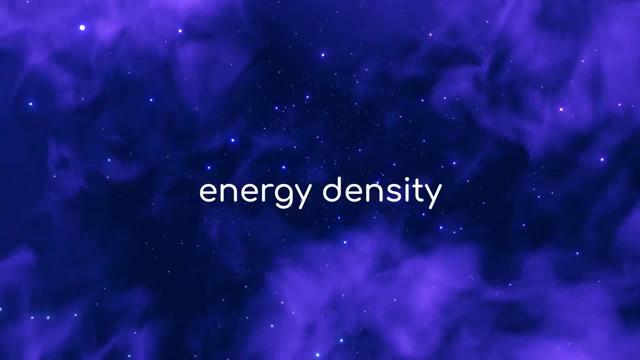 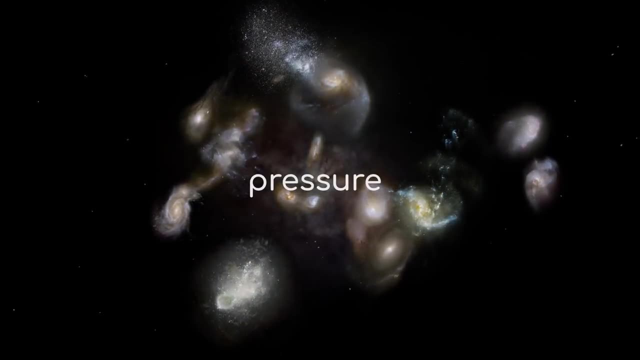 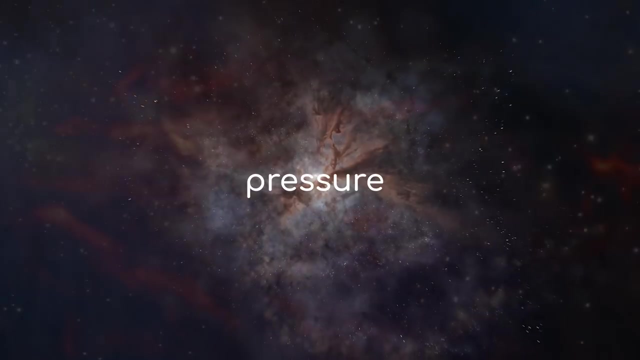 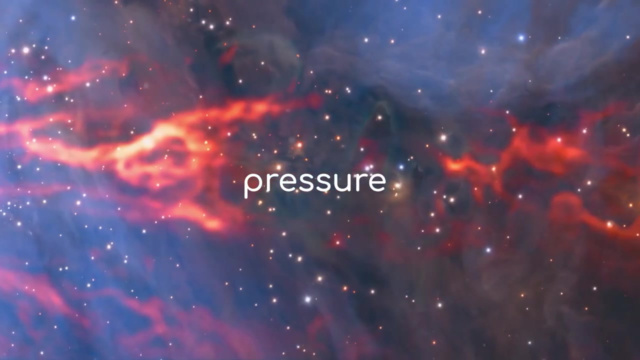 zap and motion exists within a given space ¬ ¬ in our universe has always been found to be positive. Pressure is how much force over an area the contents of that space sends pushing into the rest of the universe around it. Think interstellar dust pushing on each other whenever they bump into each other in the void As 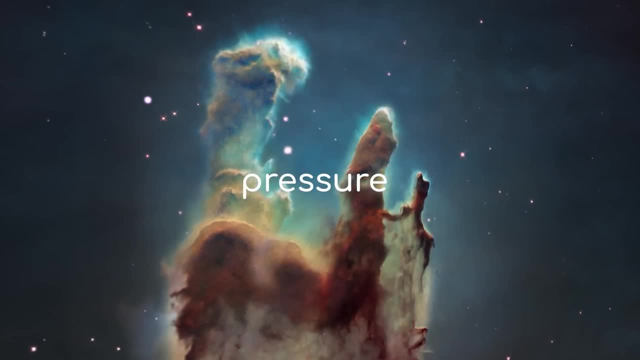 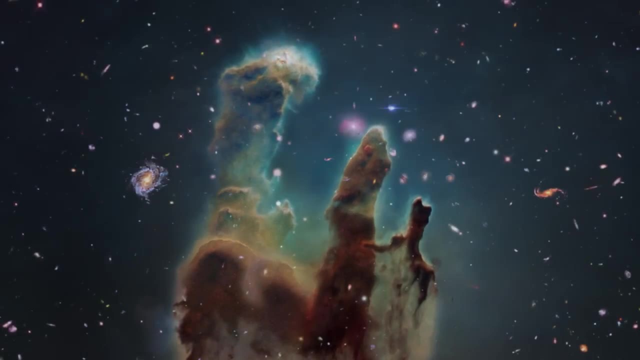 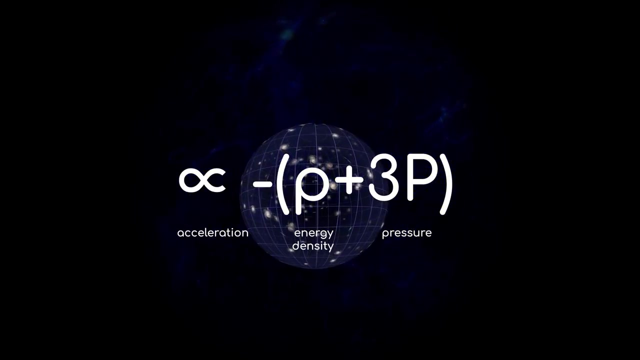 you can imagine, for objects so far apart, this pressure value hovers a little over zero on a cosmic scale. When these values are cumulatively positive, as in the following formula, their influence on the space around them causes the space around them to contract in. 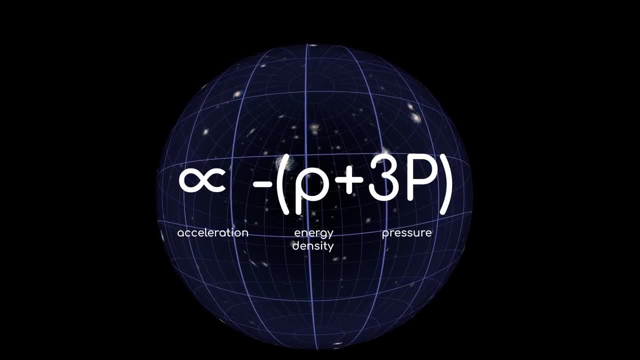 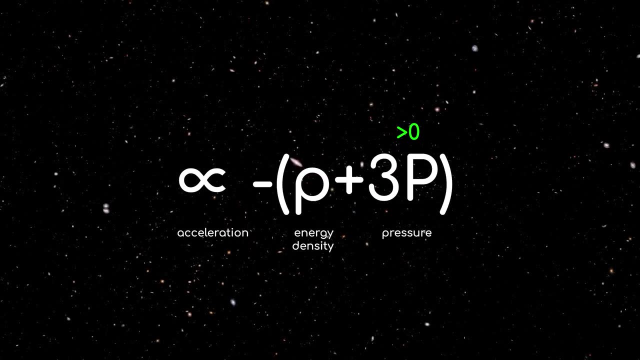 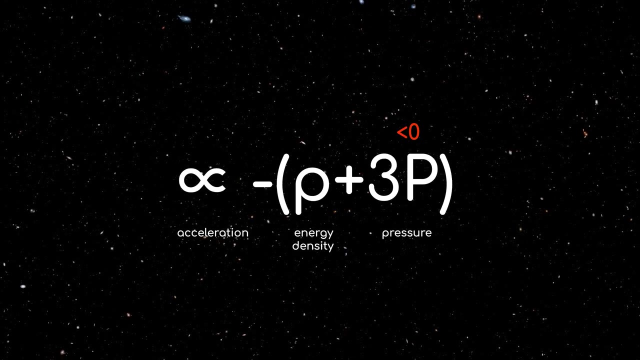 Essentially, they create gravity by decelerating the stretching of space. However, conceivably, if you were somehow to set the values of this equation so that pressure was negative and greater than the positive energy density, that minus sign would cause the whole thing to flip. 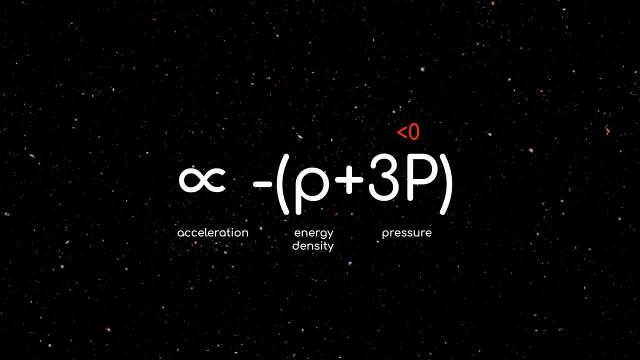 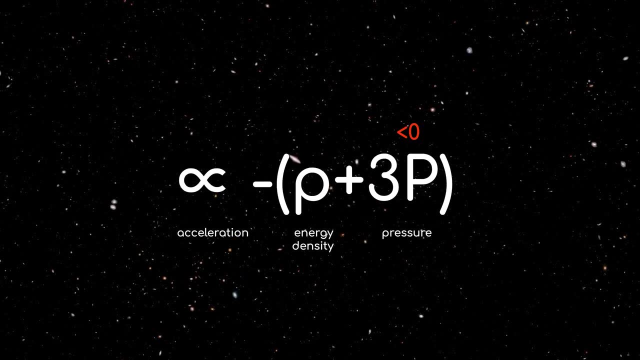 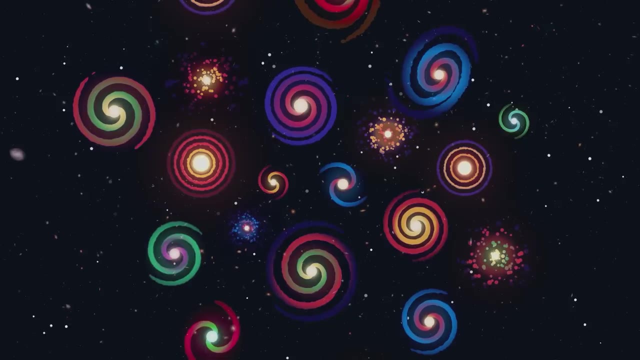 and you would accelerate the stretching of space. In effect, you would end up with a volume of space filled with a kind of anti-gravity, a dark energy. It's a little nebulous, as it's tricky to visualize anything with a truly negative pressure. How can you have less than zero atoms in a 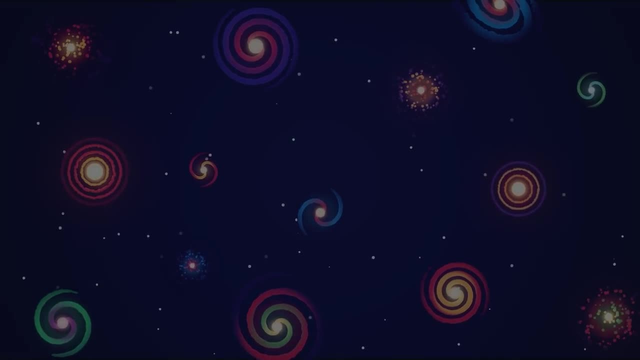 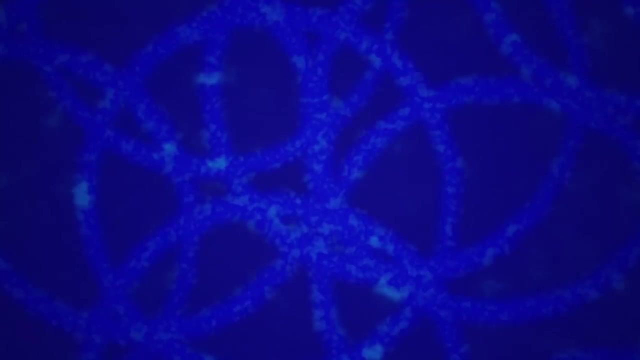 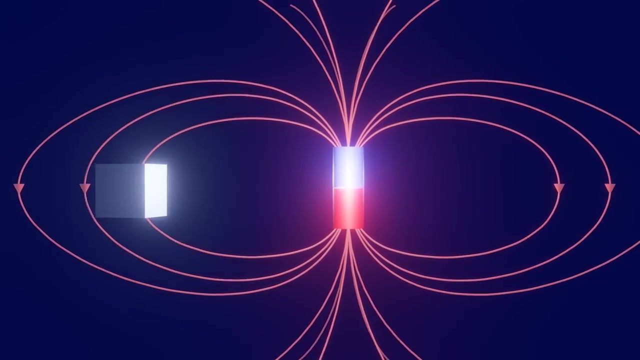 patch of space, after all. But atoms are not the only thing that exerts pressure. After all, pressure is simply a force applied across an area. Fields can also apply forces. Think a magnetic field dragging a piece of iron in towards a bar magnet, or two magnets pushing each other away. 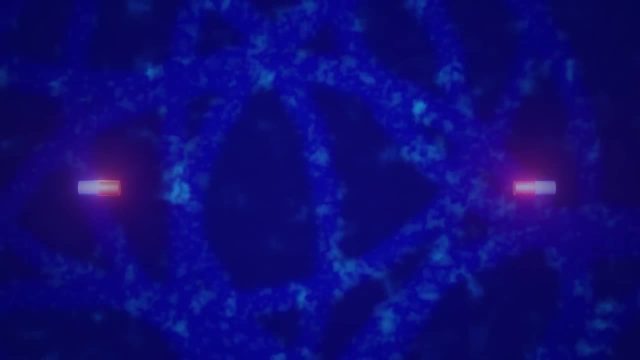 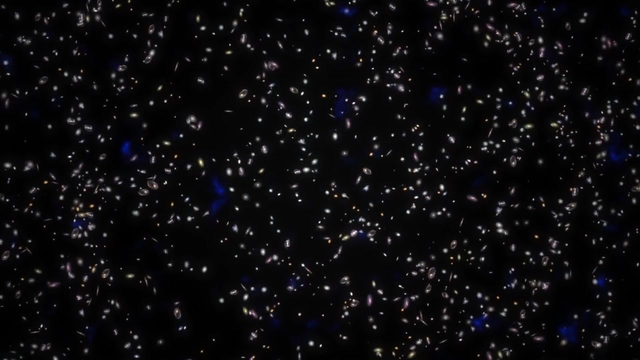 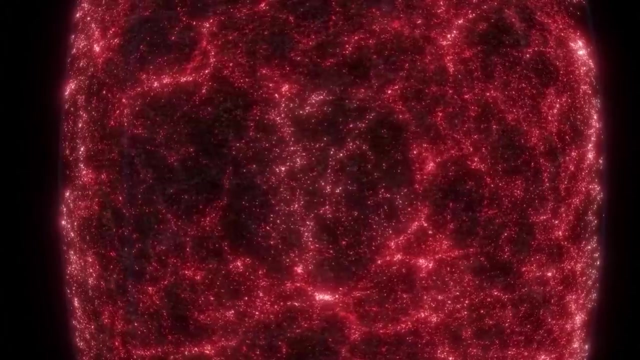 If dark energy were some kind of field that pushed away not just other magnets but everything, then this would match what we see the universe doing: Vacuum itself having dark energy and enough of it to slowly, very gently, push the universe apart. 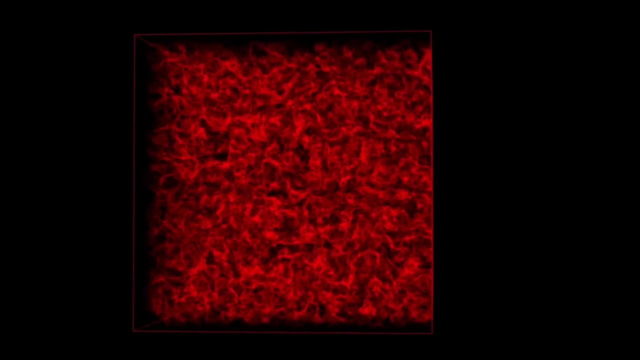 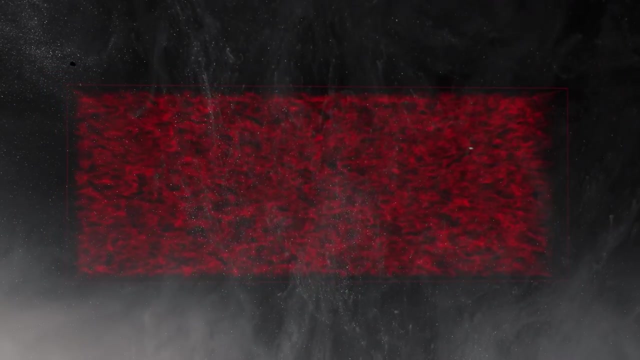 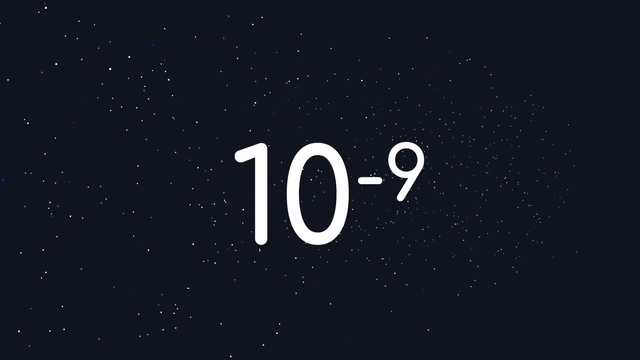 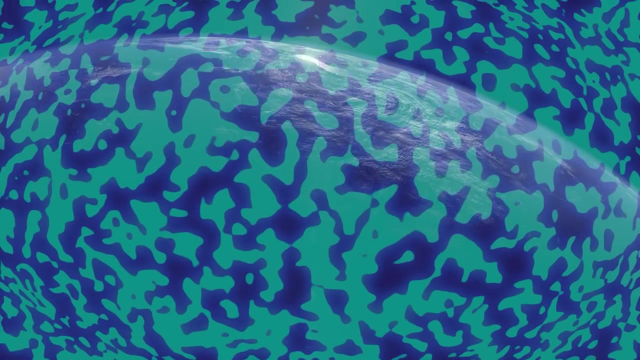 Scientists have thought a lot about dark energy over the years and have even figured out what its combined energy density and pressure needed to be to create the rate of spatial expansion that we witness. It's around 10 to the power minus 10.. This is a very small number, which is why we don't notice it here on Earth and only spot it on the 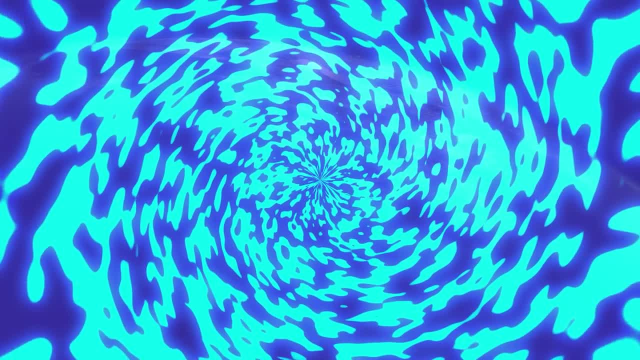 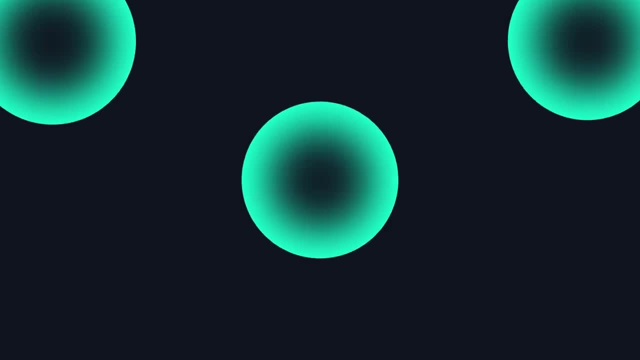 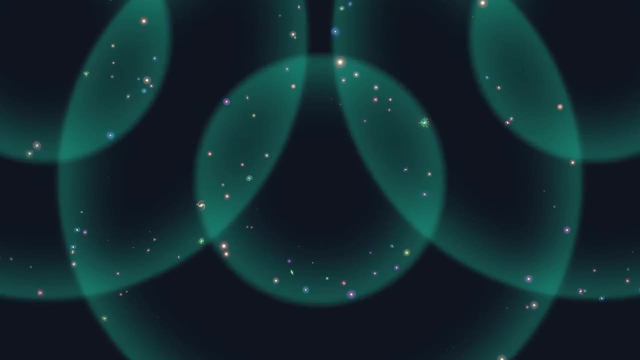 grand cosmological scale of the universe. This is actually good news, because it turns out that if the number was much higher or lower than this, things would get very bad for our chance of existing. Let me show you what I mean with a quick sketch of the history of the universe. 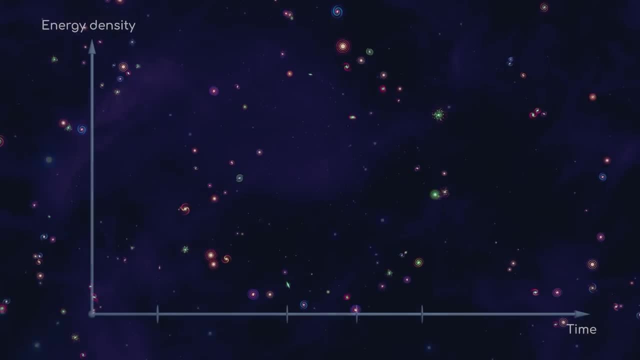 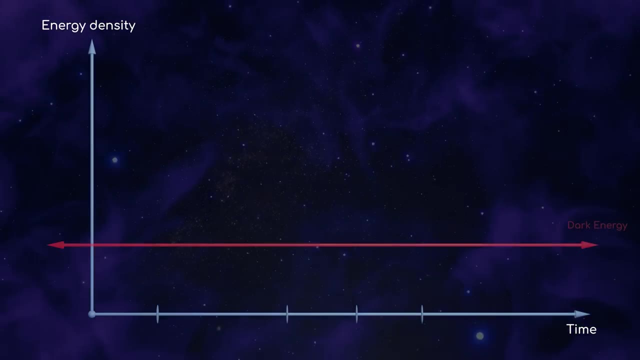 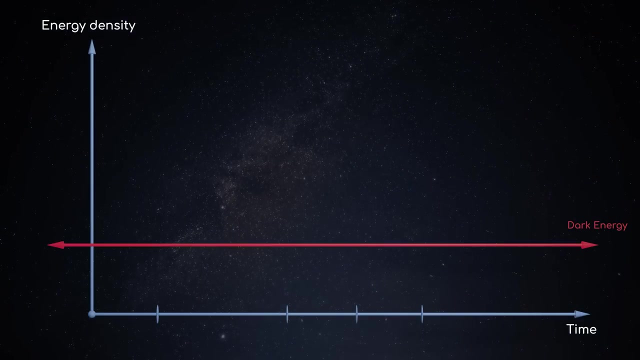 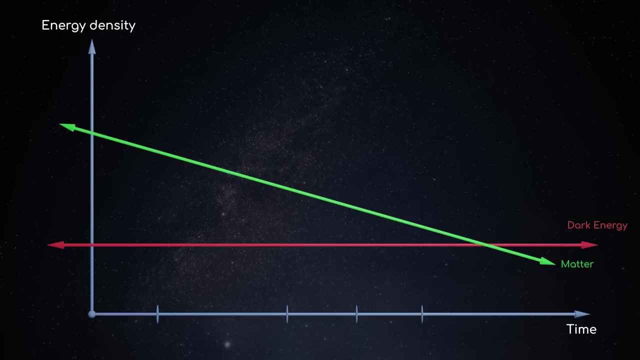 Here is the full history of the universe, from the moment just after the big bang to the present. This is the dark energy density measured by astronomers. Scientists believe its negative pressure has kept this density roughly constant for billions of years. This is the density of ordinary matter in the universe, which has little to no pressure. 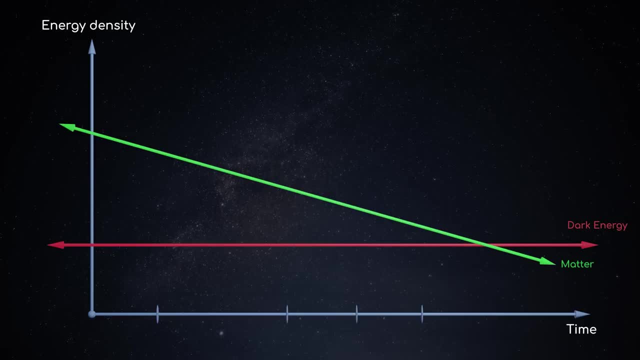 The density decreases over time because the expansion of the universe dilutes the matter within it. Finally, this is the density of radiation in the universe, including photons and other extremely light particles. The positive pressure of radiation makes it dilute away even more quickly than ordinary matter. 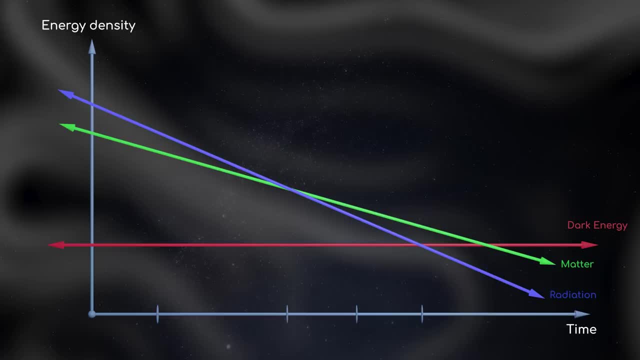 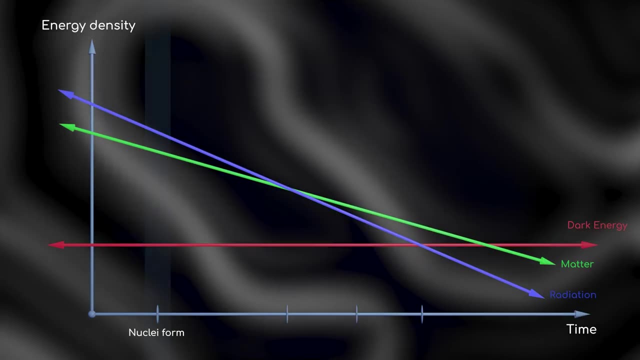 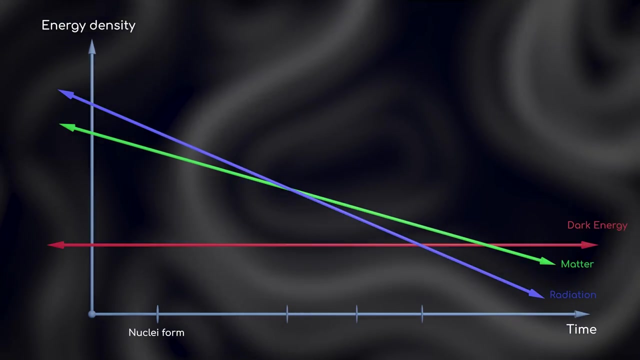 Towards the beginning of time. for a very short period there were no atoms. Very quickly, though, protons and neutrons fused together to create the first atomic nuclei in the very early universe. Shortly after matter took over as the dominant form of energy, the universe cooled down enough. 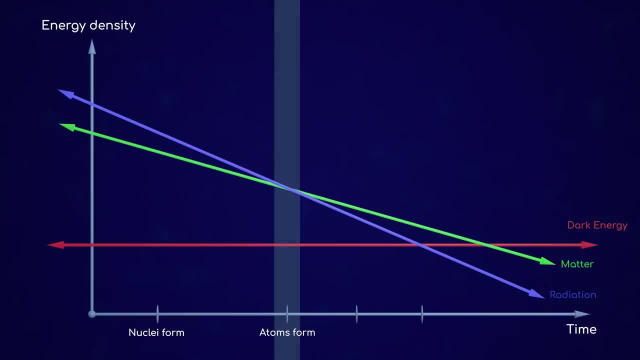 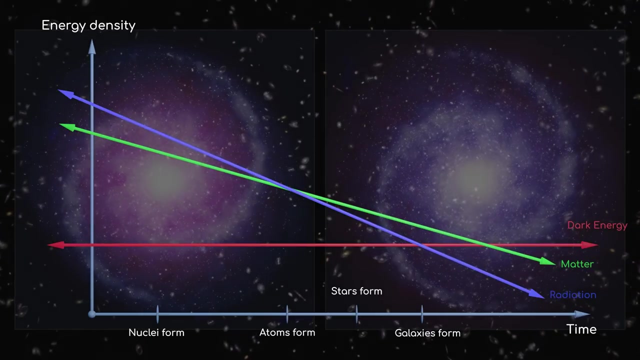 for those nuclei to attract and hold onto electrons, forming the first atoms of hydrogen and helium. These atoms were the building blocks of the very first stars, and these stars were pulled together by gravity to form the very first stars, galaxies and clusters. Only later did dark energy take over, triggering the accelerated 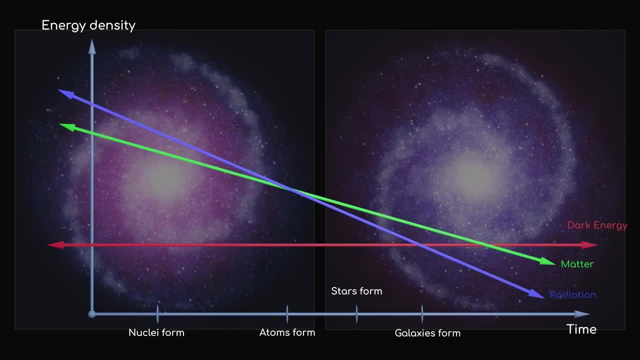 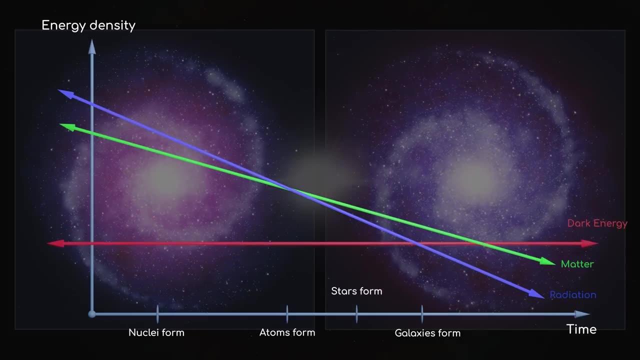 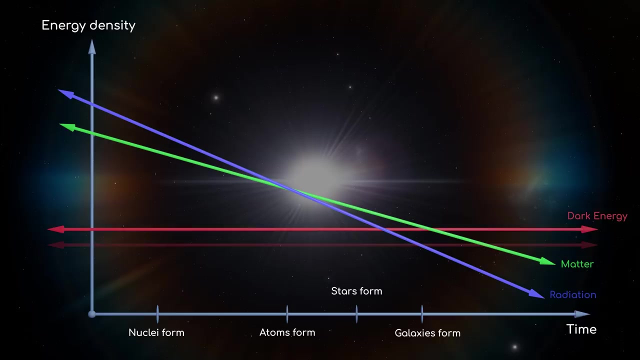 expansion of space and preventing the formation of larger structures. But what would have happened if the energy density were larger? Consider what would have happened if the pushing force of dark energy was stronger. It could have been enough to halt the formation of those early galaxies, pushing apart stars more powerful than ever before. 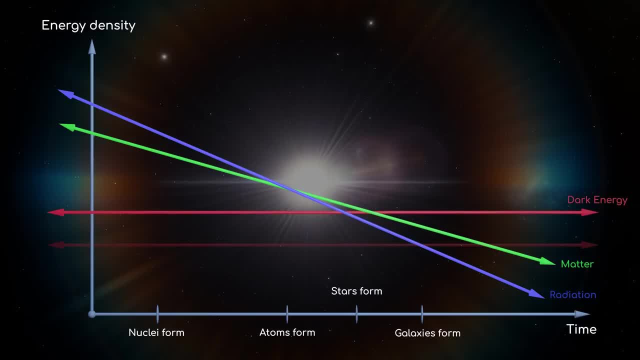 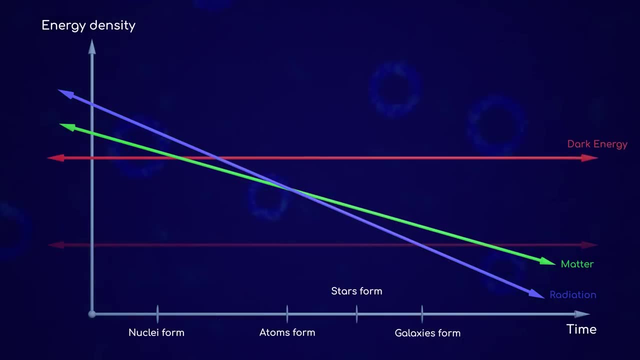 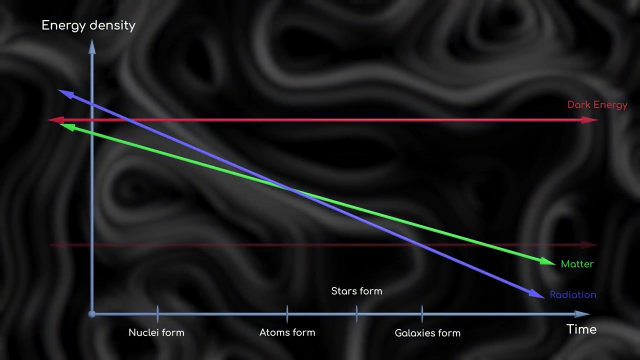 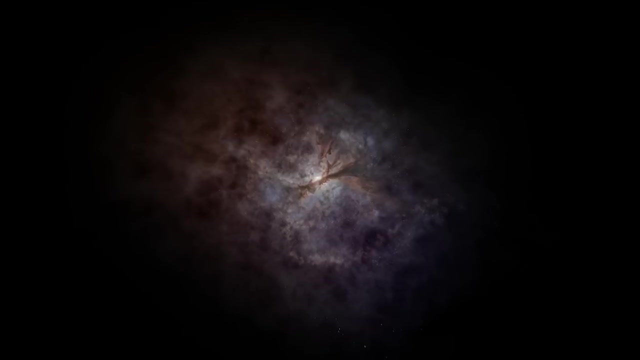 A bit larger than that, and it would have been much more difficult for any stars to form either. And if the dark energy density were large enough, we would hardly have had any atoms or even nuclei produced in the universe. So that's what it could have been. What should it have been? 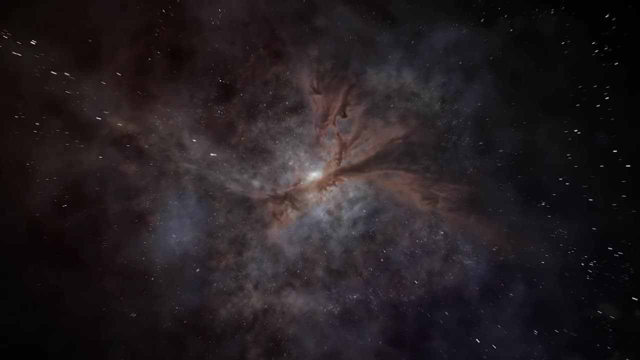 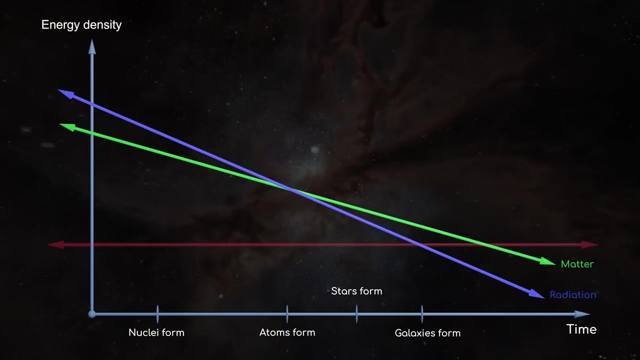 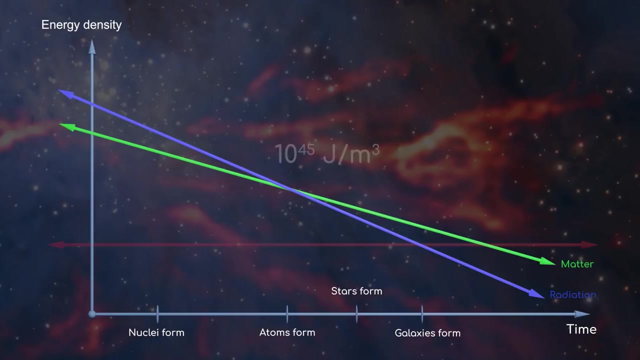 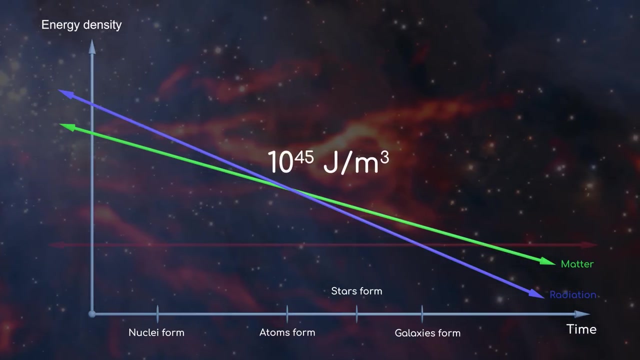 Using some clever maths and the principles of quantum field theory, scientists attempted to predict how much the energy density of dark energy ought to have been. Their result was larger than the result we see in nature. How much larger Their value came in at an astounding 10 to the power, 45 joules per cubic metre. 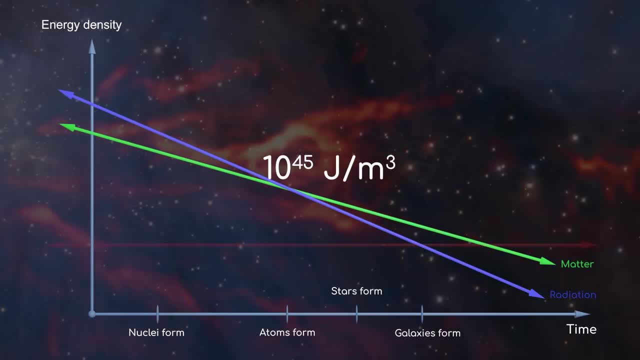 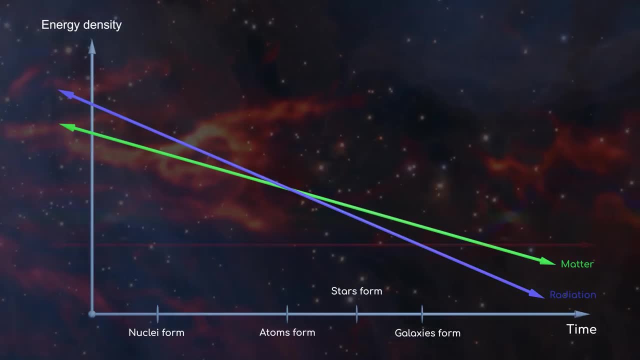 So where does the predicted energy density of 10 to the power- 45 joules per cubic metre fall on this graph? So where does the predicted energy density of 10 to the power- 45 joules per cubic metre- fall on this graph? It's quite literally off the charts. If that prediction were correct, the universe today 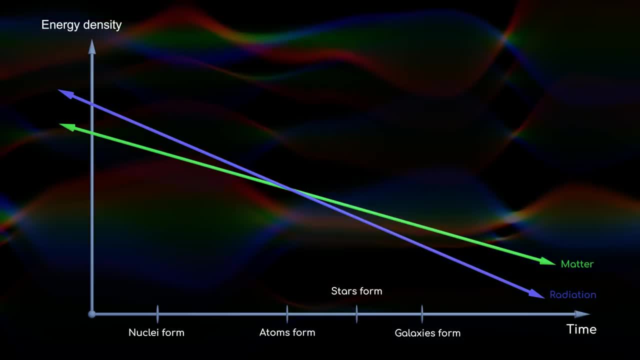 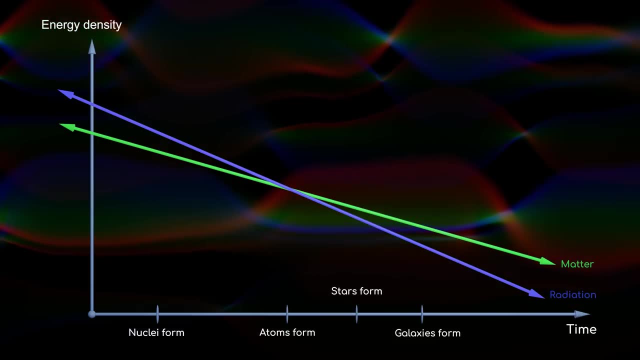 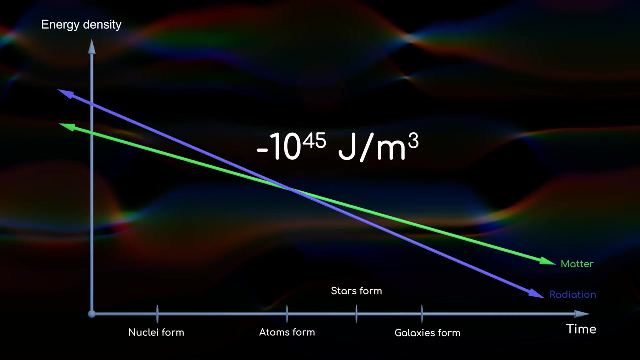 would have no structure, no features, no life. It would be a giant void filled with nothing but dark energy. And if the dark energy density were instead a negative 10 to the power, 45 joules per cubic metre, the fate of the universe would be no more promising, as it would be forced to. rapidly collapse in on itself. So if the dark energy density were instead a negative 10 to the power, 45 joules per cubic metre, the fate of the universe would be no more promising, as it would be forced to rapidly collapse in on itself. So if the dark energy density were instead a negative 10 to the power- 45 joules per cubic metre- the fate of the universe would be no more promising, as it would be forced to rapidly collapse in on itself. So if the dark energy density were instead a negative 10 to the power- 45 joules per cubic metre- the fate of the universe would be no more promising, as it would be forced to rapidly collapse in on itself. 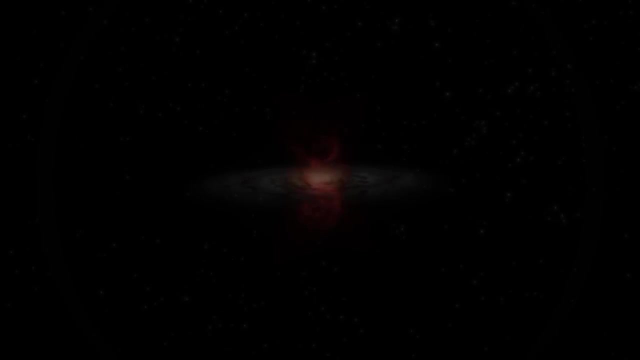 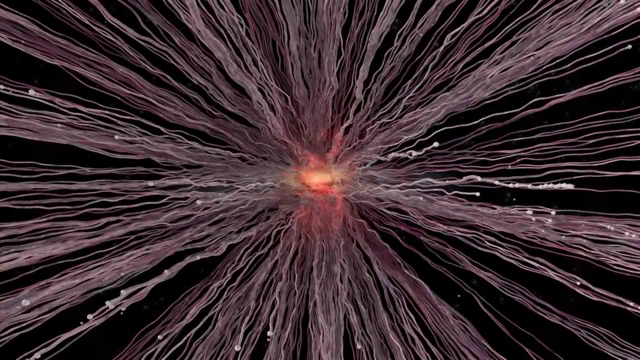 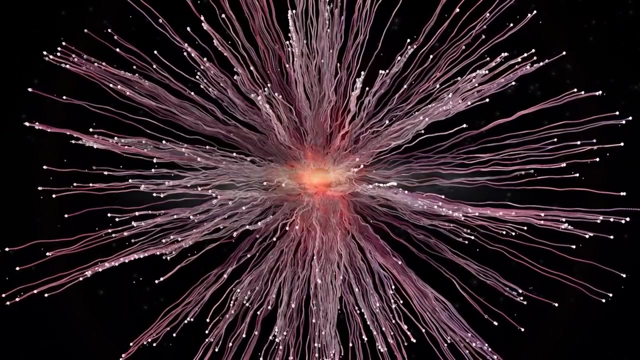 In what's known as a Big Crunch. Scientists have attempted to account for their number being so far off by hypothesizing that there exists particles with positive energy and negative pressure as yet undiscovered. that even out the maths and brings the answer for dark energy density back down towards. 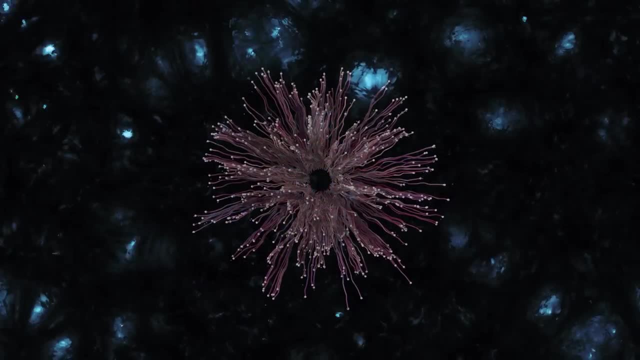 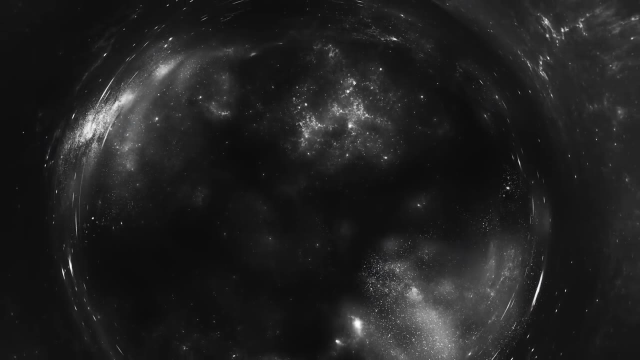 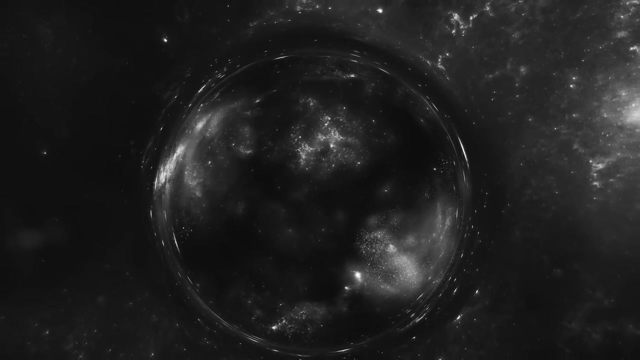 zero. Perhaps there is some massive negative potential energy source that evens all the maths out, a cosmic stretched spring that somehow reigns in all that rampant energy. Either that or quantum field theory is fundamentally wrong. But as there's actually quite a lot of evidence supporting quantum field theory, 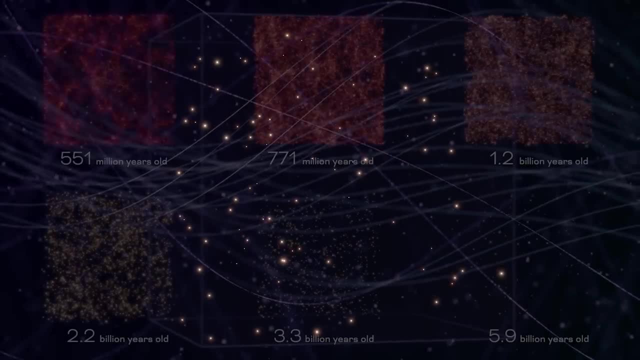 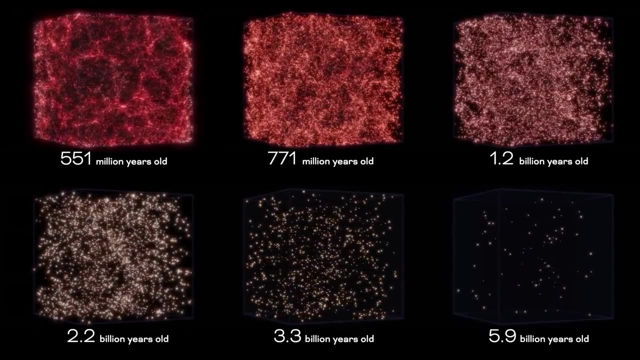 it seems imprudent to completely throw the idea out. Instead, we are left contemplating the marvellous nature of this cosmic coincidence. What were the odds that the energy density of dark energy would be so low when it was predicted to be so much higher? 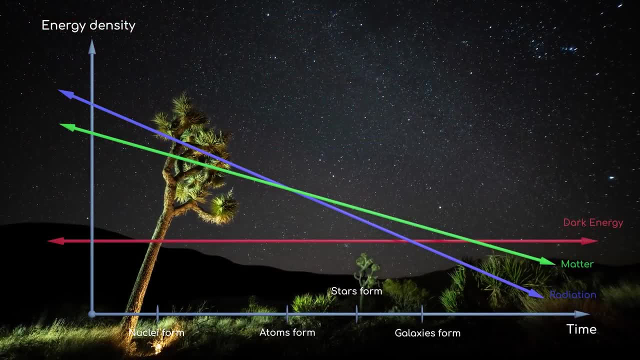 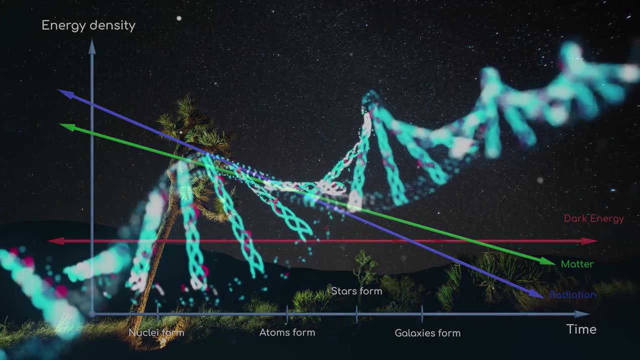 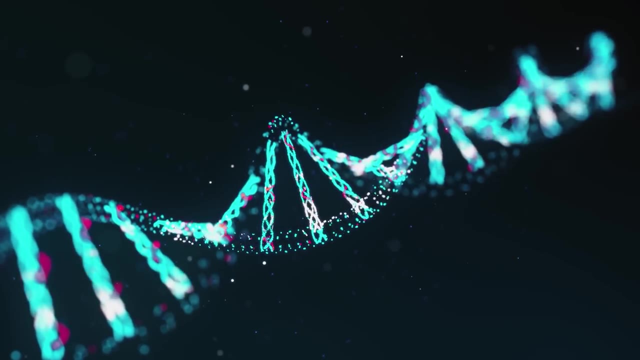 That this great universal balancing act occurred in such a way that we weren't torn apart or crushed into a singularity. Without it being so low in magnitude, we wouldn't exist. Our very atoms would have never come together, torn apart by surging, expanding space. 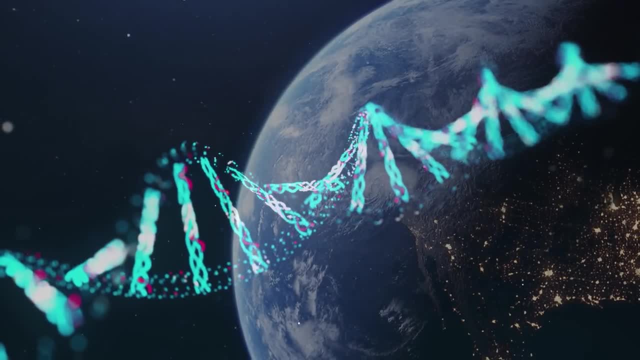 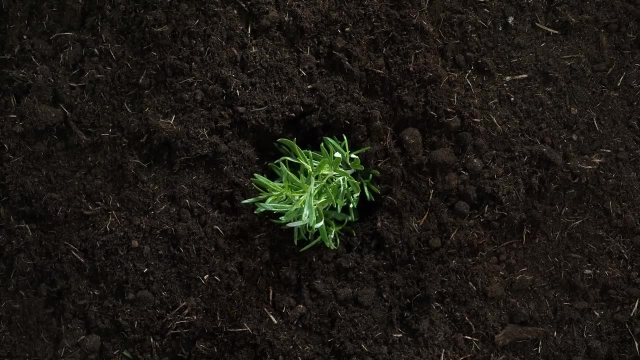 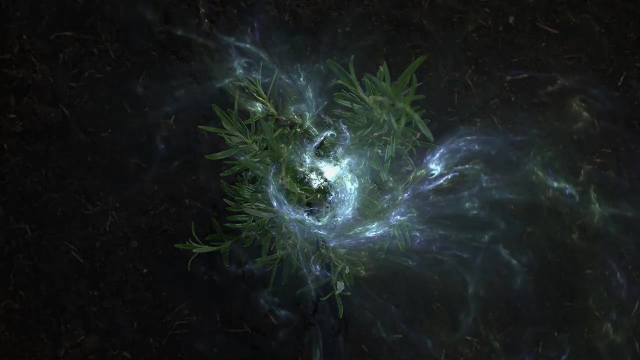 According to our predictions, we have got very lucky. This coincidence happened in such a way that the universe was able to produce life. So was it a coincidence? The answer to that question strays from what we know for sure into what we simply theorise, however. 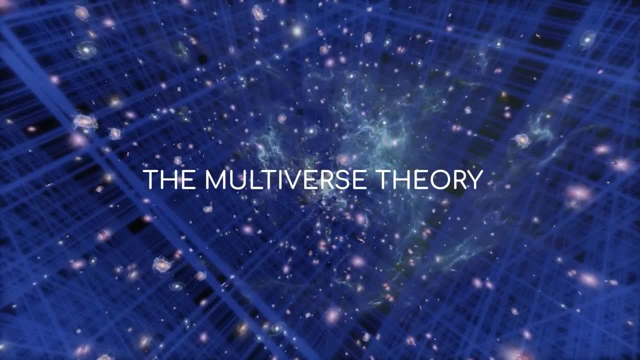 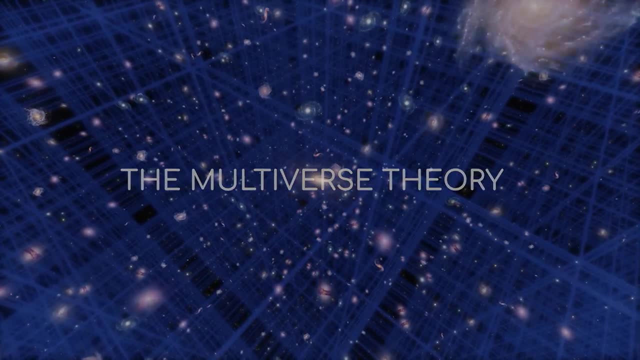 It wanders into the realms of multiverse theory and mankind's quest to understand if we are not here by chance but by design. There's a lot to cover, too much to cram into the end of this video, and so, to do it justice, I've split this one into two. 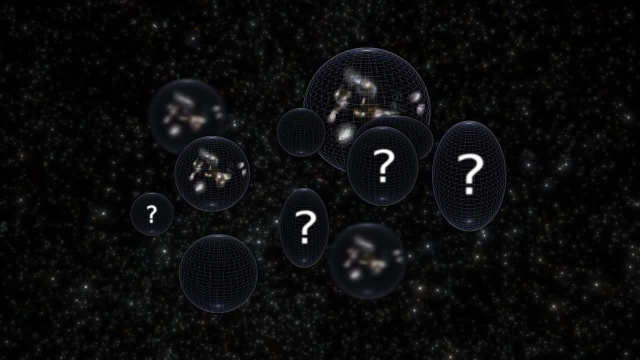 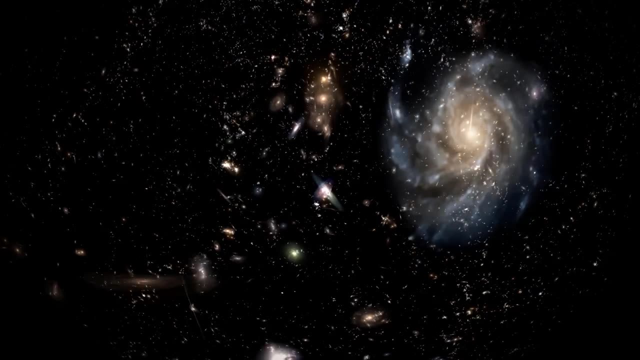 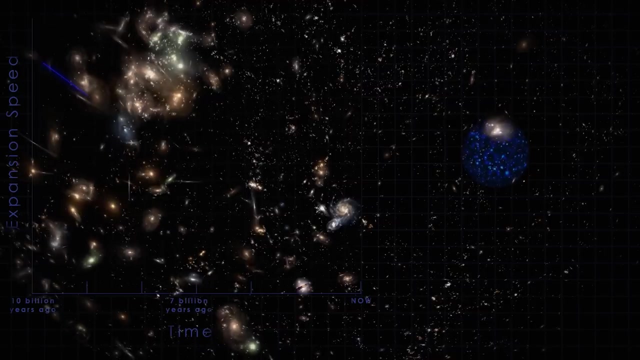 I'll cover the rest when I have the time to do it full justice. In the meantime, what do you think? Our existence so far appears to be excessively fortunate. How do you think it happened? Leave your answer in the comments below and see if other people's ideas match or contrast with your own. 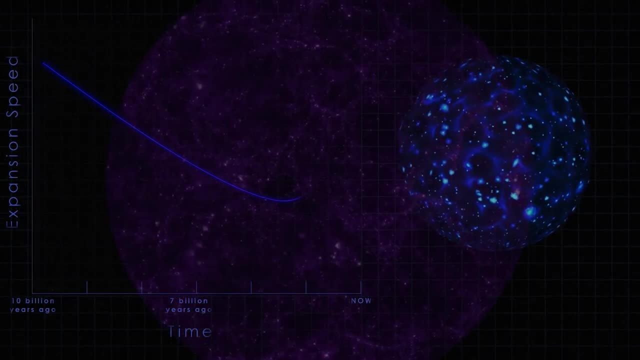 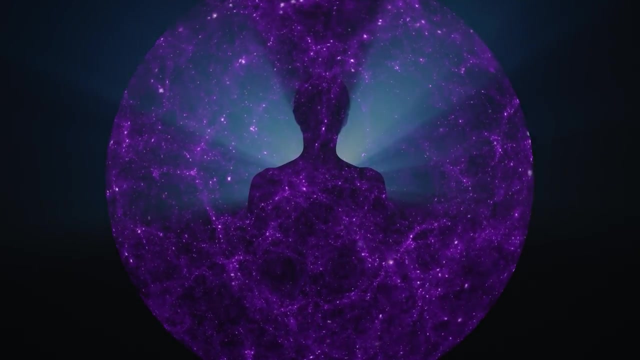 It's always good to know. It's always good to hear from other viewpoints, particularly for a subject where there aren't clear-cut answers. You never know what you might find out. Our existence is surprising. Perhaps that means the universe has more surprises in store for us if we can only find the answers. 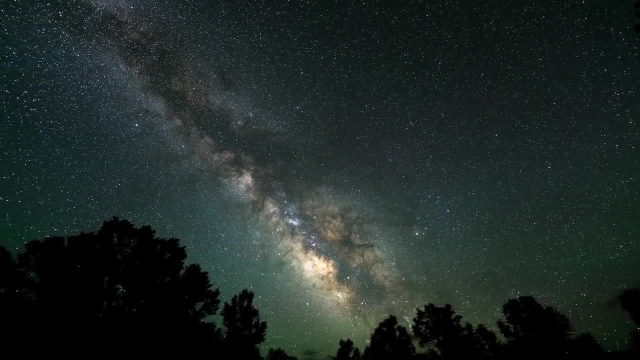 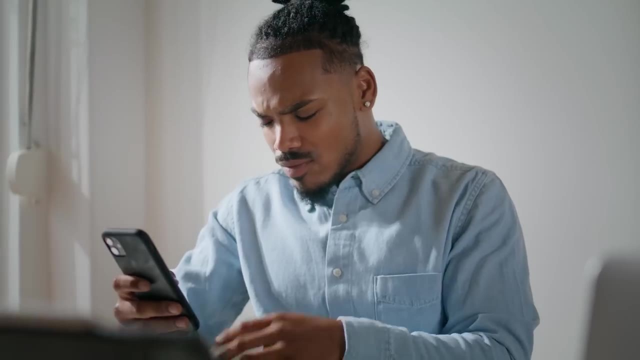 Figuring out how the universe came to exist is a complicated task. There are a lot of moving parts, new discoveries that evolve our understanding and intricate mathematics to get to. But it's not all about the answers. There are a lot of things that you can do to change your head around. 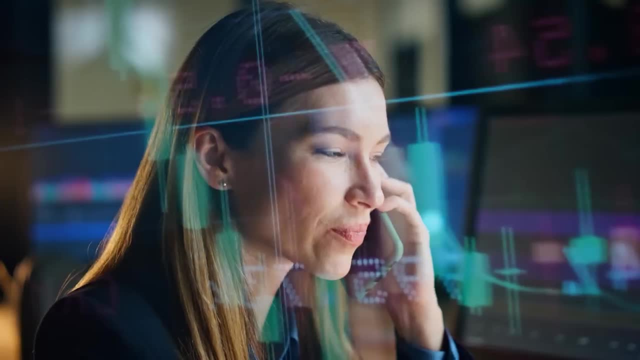 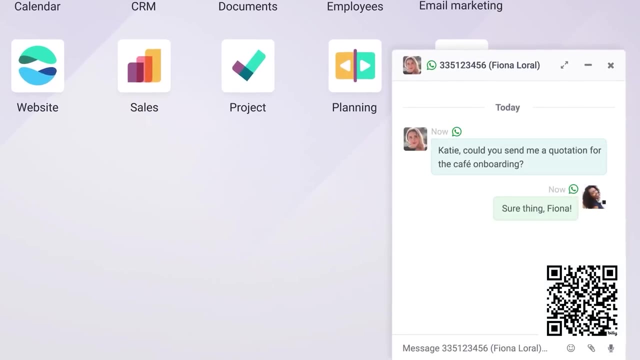 No wonder we don't have all the answers yet. Thankfully, running a business doesn't have to be quite so complicated, thanks to the sponsor of today's video, Odoo. Odoo is a business platform that has all the apps you need to run a business. 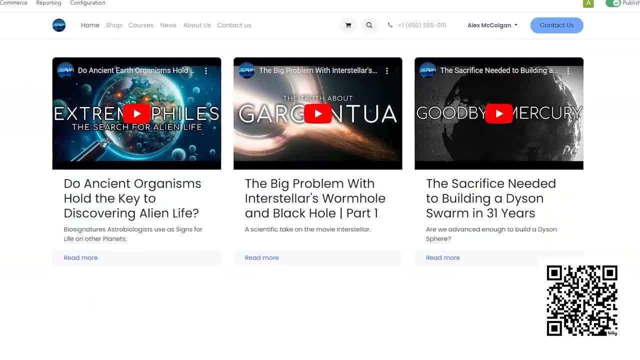 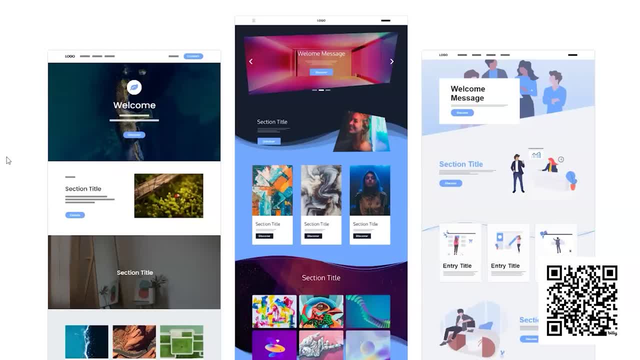 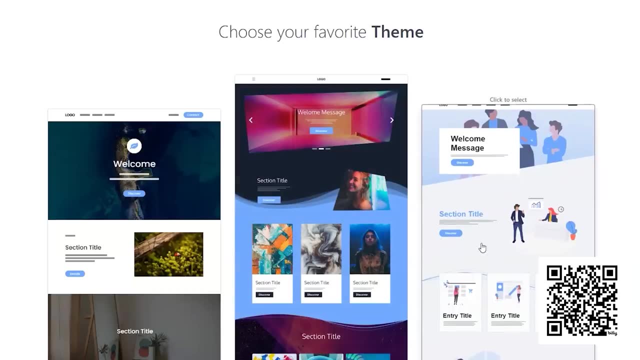 from sales to accounting to building a website. The best part is they're all connected. Getting a document signed in one app will instantly update the others. Their website builder was one of the apps that drew my attention most. It's incredibly easy to make and edit a website from scratch with just four little steps. 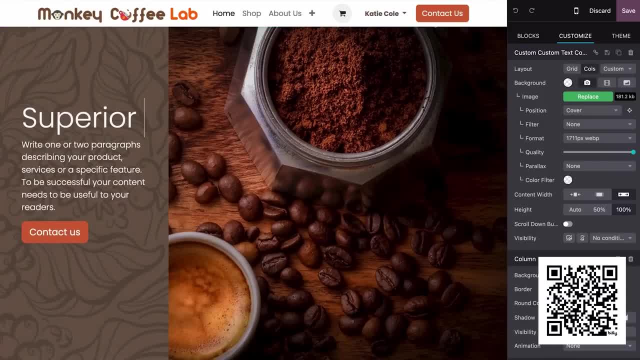 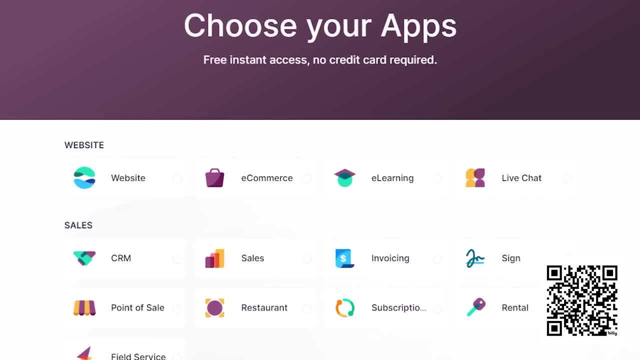 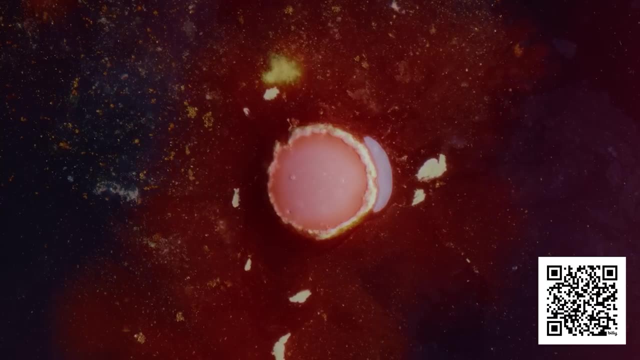 Drag and drop some blocks, just edit text, colours and pictures. Everything is fully customisable. Odoo's first app is completely free forever, such as the website builder, and this all comes with free support and unlimited hosting. Scan my QR code or click my link in the description below. 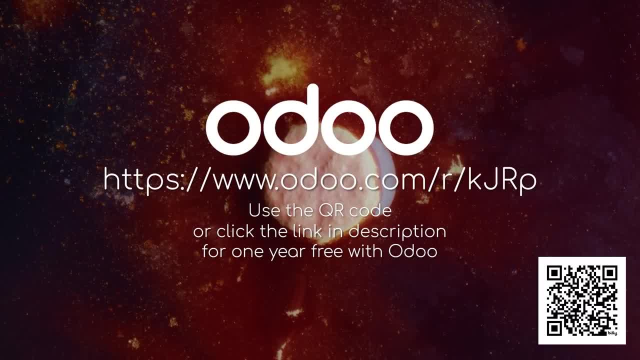 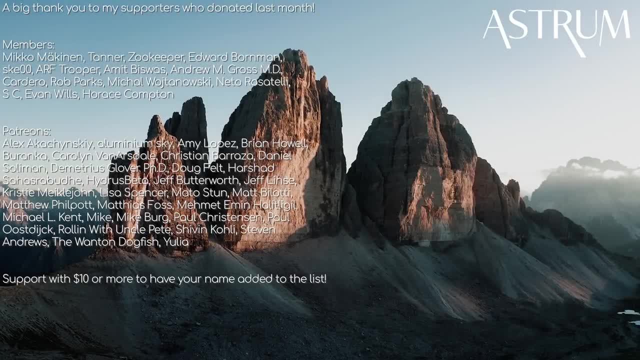 and gain access to your one year free custom domain that Odoo is giving away. Go on, give it a try. Thanks for watching. If you like imagery-based videos, you may like my others in this playlist. A big thanks to my patrons and members. 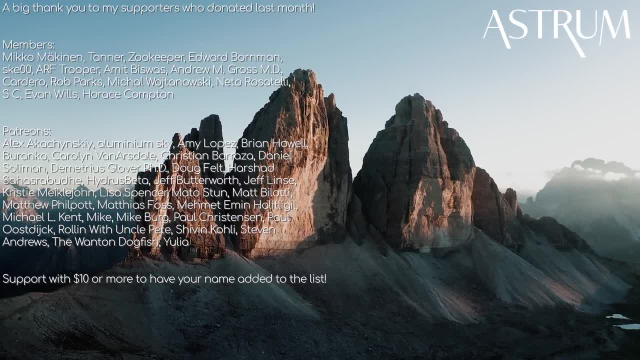 If you want to support and have your name added to the end of every Astrum video, check the links below. All the best and see you next time.